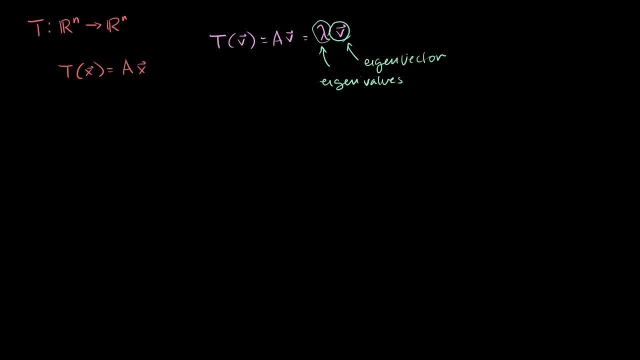 little bit of appreciation of why they're useful. But now in this video, let's at least try to determine what some of them are. You know, based on what we know so far. if you show me an eigenvector I can verify that it definitely is the case. 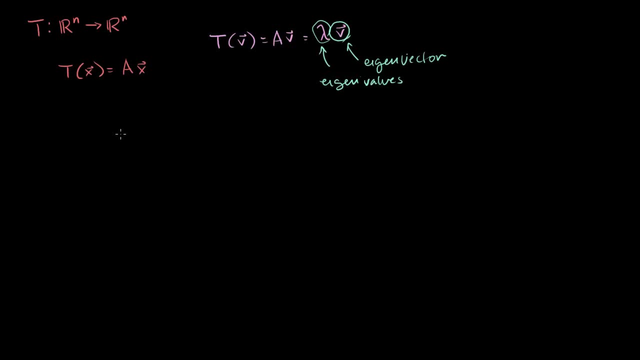 Or an eigenvalue. I could verify the case, But I don't have a systematic way of solving for either of them, So let's see if we can come up with something. So, in general, we're looking for solutions to the equation. 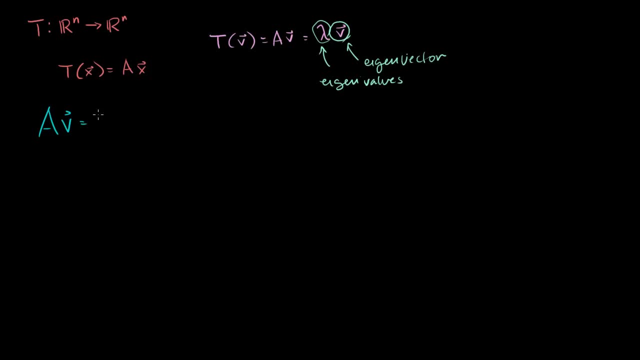 a times v is equal to lambda v. It's equal to lambda times the vector. Now one solution might immediately pop out at you, And that's just: v is equal to the 0 vector And that definitely is a solution, Although it's not normally considered to be an. 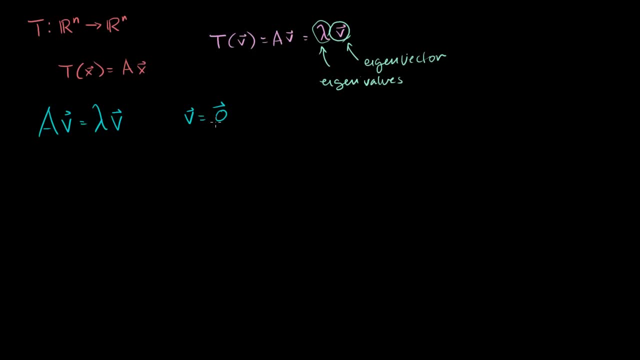 eigenvector Just because one. it's not a useful basis vector. It doesn't add anything to a basis. It doesn't add you know really the amount of vectors that you can span when you throw the basis vector in there. 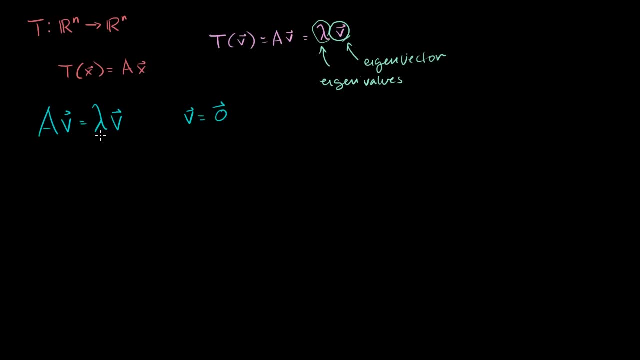 And also it's not clear what is your eigenvalue that's associated with it, Because if v is equal to 0, any eigenvalue will work for that. So normally when we're looking for eigenvectors, we start with the assumption that we're looking for non-0 vectors. 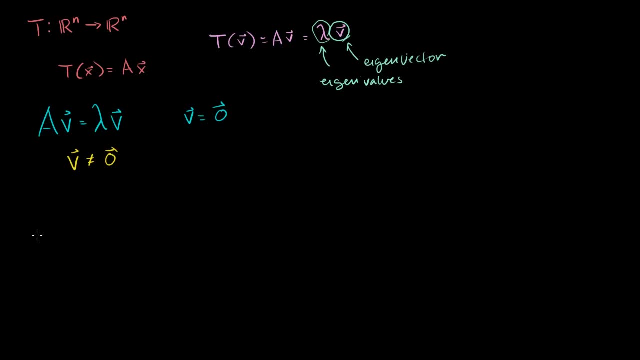 So we're looking for vectors that are not equal to the 0 vector. So, given that, let's see if we can play around with this equation a little bit And see if we can at least come up with eigenvalues, maybe in this video. 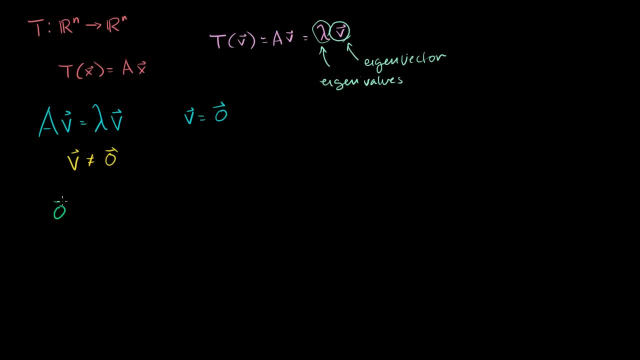 So we subtract a v from both sides, We get the 0 vector is equal to lambda v minus a times v. Now we can rewrite v as v is just the same thing as the identity matrix times v. right v is a member of Rn. 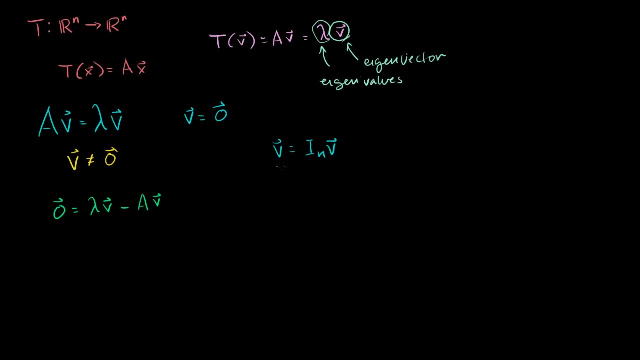 The identity matrix n by n, you just multiply, We're just going to get v again. So if I rewrite v this way, at least on this part of the expression, and let me swap sides, so then I'll get lambda times. instead of v I'll write the identity matrix, the. 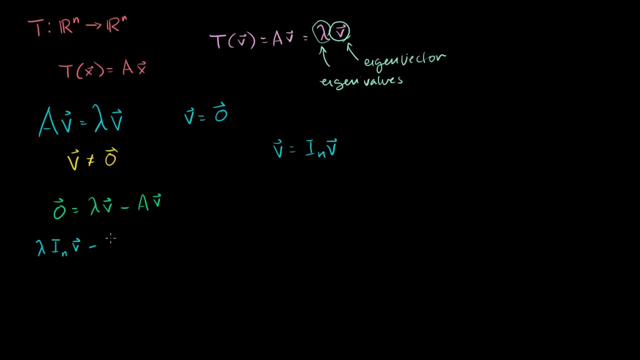 n by n. identity matrix times v minus a times v is equal to the 0 vector. Now I have one matrix times v minus another matrix times v, Matrix vector products. they have the distributive property, So this is equivalent to the matrix lambda times the. 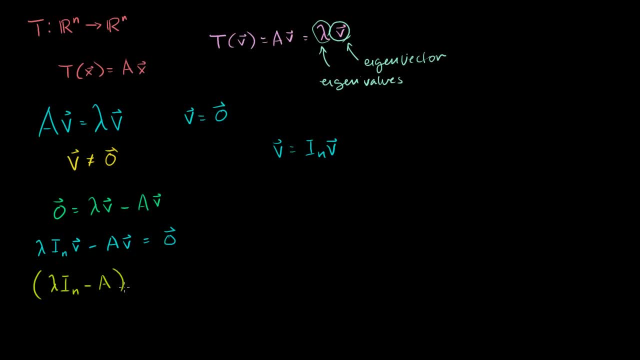 identity matrix minus a, And that's going to be equal to 0, right, This is just some matrix. right here, some matrix. And the whole reason why I made this substitution is so that I could write this as a matrix vector product instead. 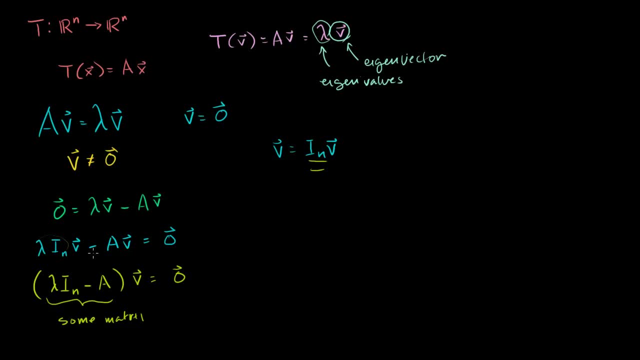 of just a scalar vector product, And that way I was able to essentially factor out the v and just write this whole equation, as essentially some matrix vector product is equal to 0.. Now, in order, if we assume that this is the case- and we're assuming, remember we're 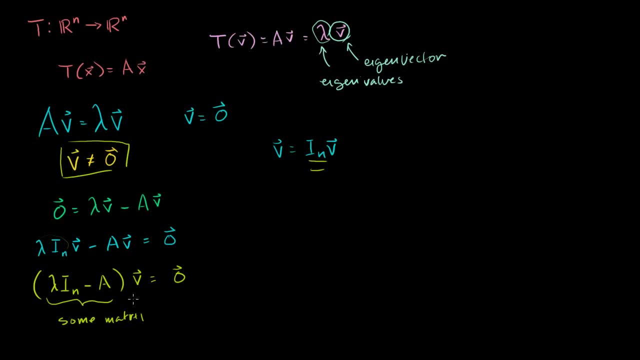 assuming that v does not equal to 0,. so what does this mean? So we know that v is a member of the null space of this matrix. right here Let me write this down: v is a member of the null space of lambda. i, sub n minus a. 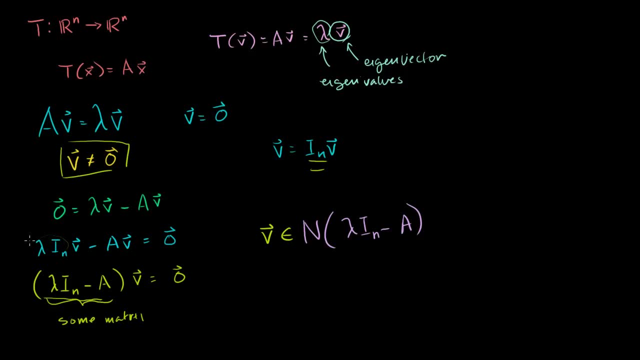 I know that might look a little convoluted to you right now, but just imagine this is just some matrix B. It might make it simpler. This is just some matrix here. right, That's B. Let's make that substitution. Then this equation just becomes: Bv is equal to 0.. 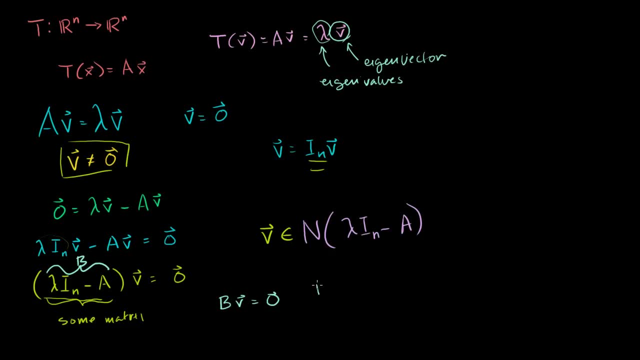 Now, if we want to look at the null space of this, the null space of B is all of the vectors x that are a member of Rn, such that B times x is equal to 0.. Well, v is clearly one of those guys, right. 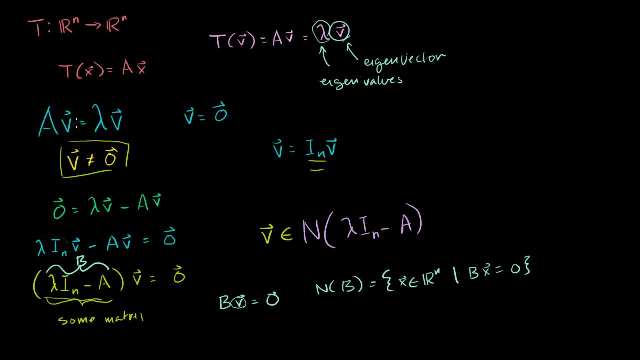 Because B times v is equal to 0. We're assuming v solves this equation and that gets us all the way to the assumption that v must solve this equation And v is not equal to 0. So v is a member of the null space and this is a. 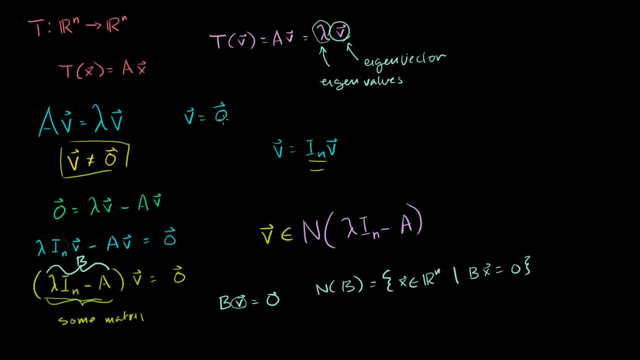 nontrivial member of the null space. We already said that the 0 vector is always going to be a member of the null space and it would make this true. But we're assuming v is non-zero, We're only interested in non-zero eigenvectors and that. 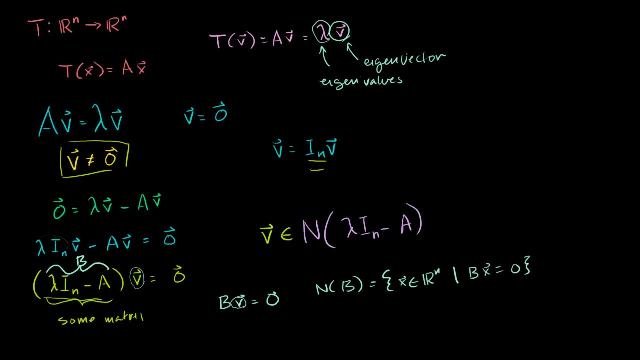 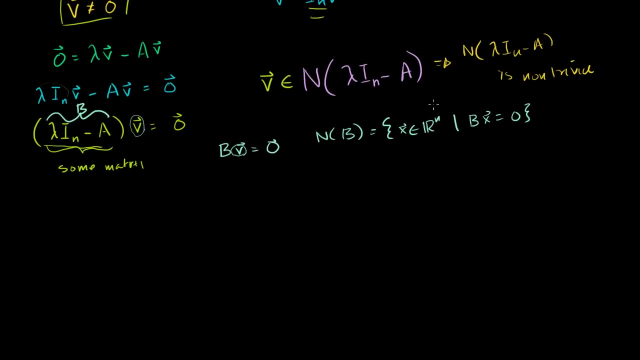 means that this guy's null space has to be nontrivial. So this means that the null space of lambda in minus a is nontrivial. The 0 vector is not the only member. You might remember before that, the only time we write this in. 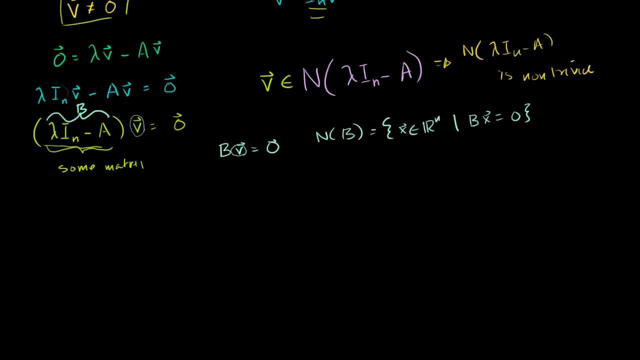 general, if I have some matrix- I don't know I've all used a and b. let's say I have some matrix D. D is d's. D's columns are linearly independent if, and only if, the null space of d only contains the 0 vector. 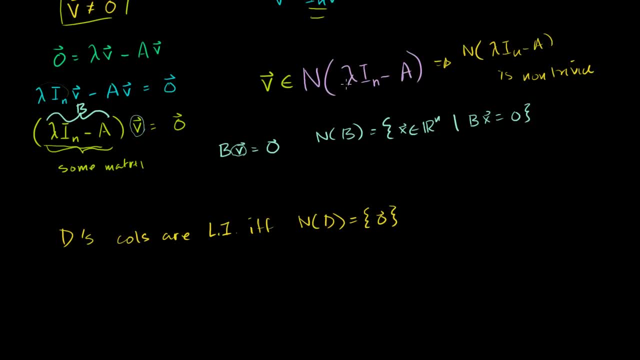 So if we have some matrix here whose null space does not only contain the 0 vector, then it has linearly dependent columns. So we know that and I just wrote that there to kind of show you what we do know and the fact that this one doesn't. 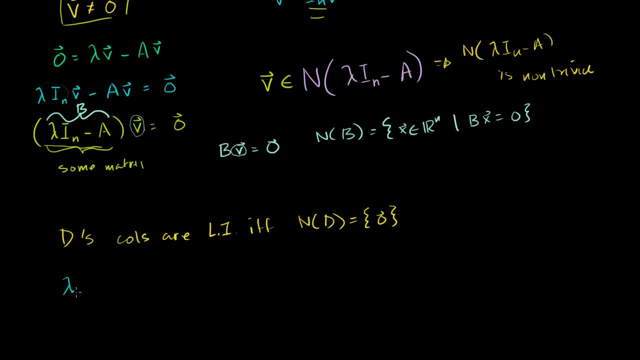 have a trivial null space tells us that we're dealing with linearly dependent columns. So lambda in minus a. it looks all fancy, but this is just a matrix. must have linearly dependent columns, Or another way to say that is: if you have linearly dependent 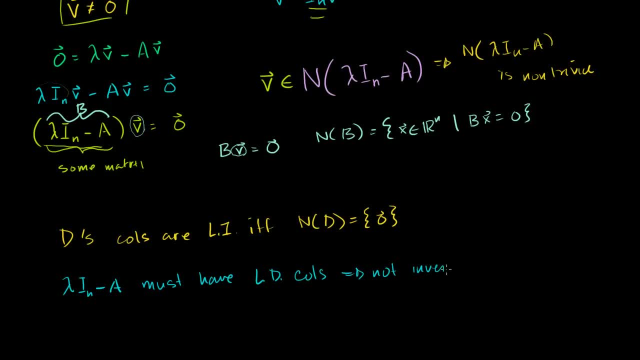 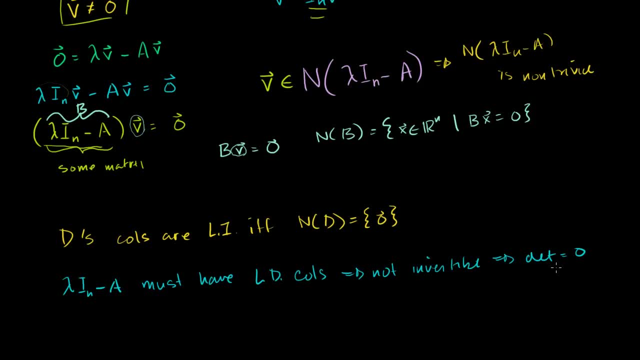 invertible. You're going to have linearly dependent columns. If your determinant is equal to 0, then that also means that you have non-trivial members in your null space, And so if your determinant is equal to 0, that means there's. 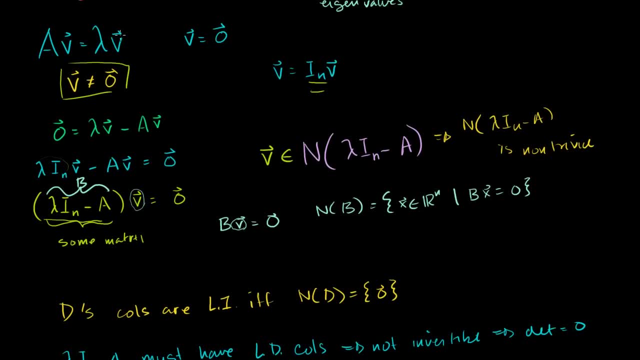 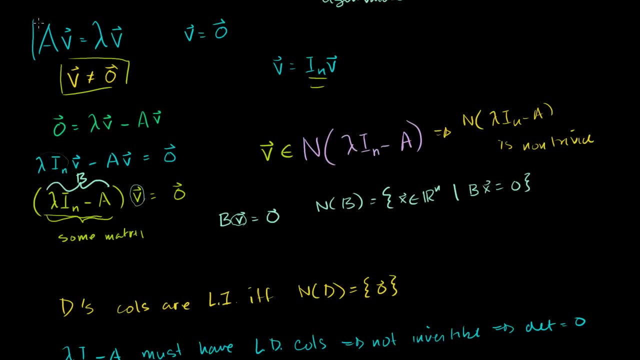 some lambdas for which this is true for non-0 vectors v. So If there are some solutions, if there are some non-0 vector v's that satisfy this equation, then this matrix right here must have a determinant of 0.. 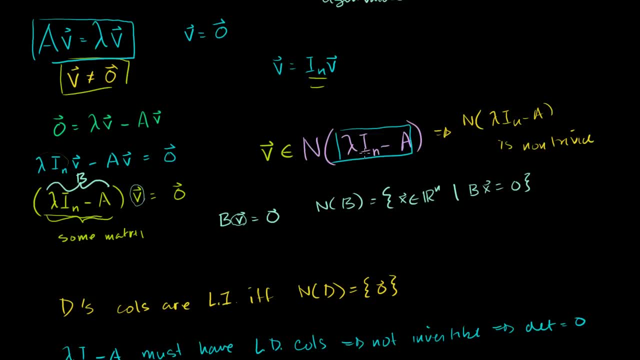 And it goes the other way. If this guy has a determinant of 0,, then there must be, or there's some lambdas that make this guy have a determinant of 0, then those lambdas are going to satisfy this equation And you can go the other way.